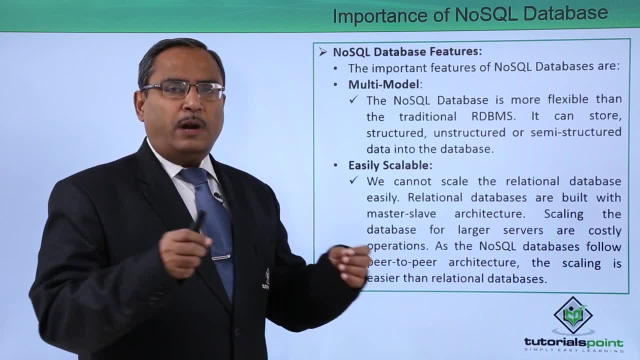 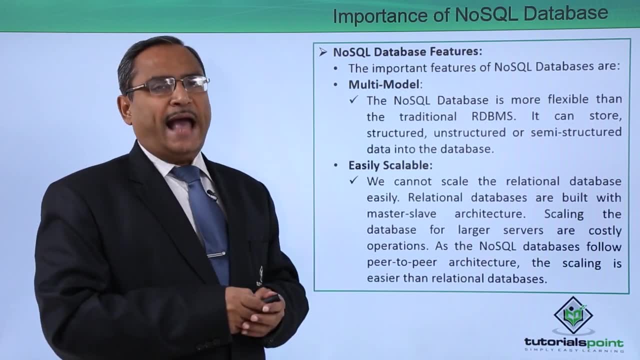 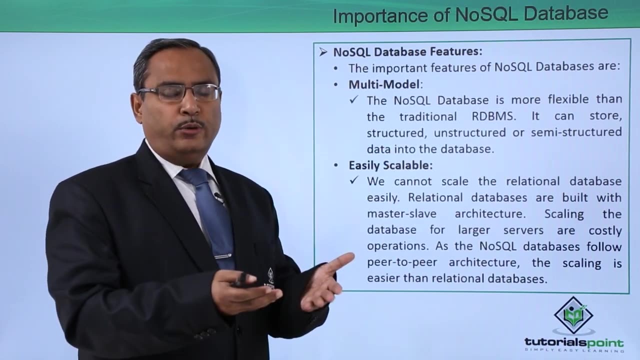 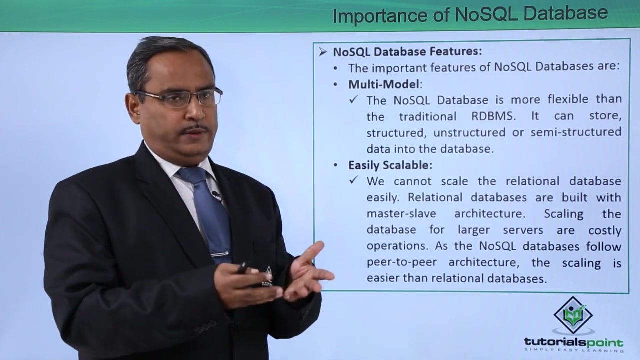 In our RDBMS we can represent our data into multiple rows and columns, and all the tables must have a static structure. But in case of NoSQL, we can have the dynamic structure here. So that is the main advantage, And it can store structured data. that means the data of whatever you are going to get from different machines, from different sensors and so on. We are having this unstructured data, that means the data in the form of images, in the form of videos, And we are having the semi-structured data, that means the data in the form of images, in the form of videos. 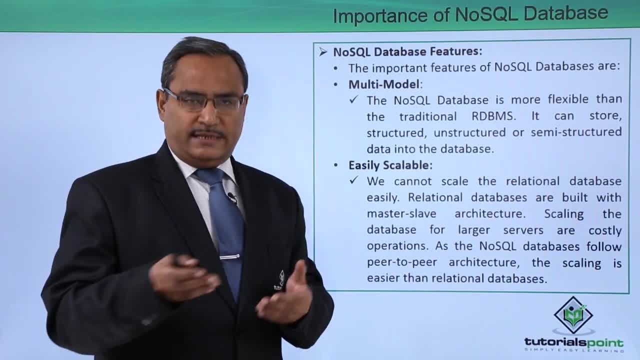 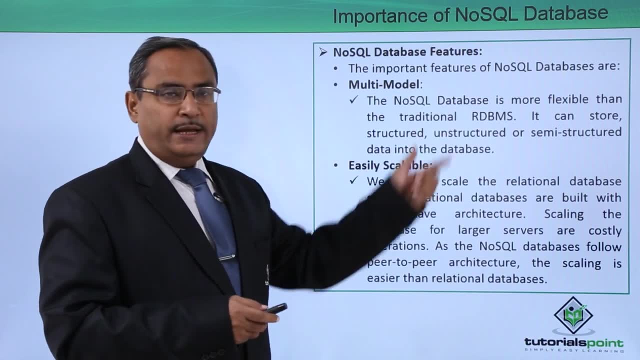 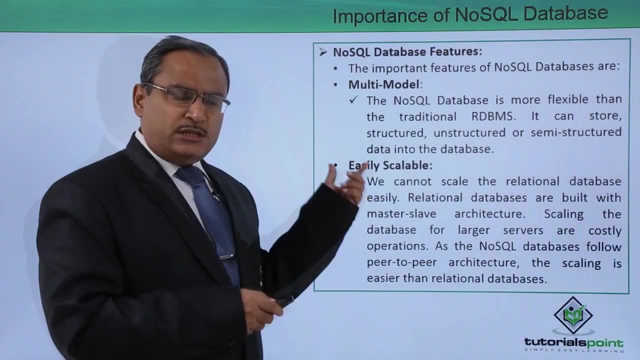 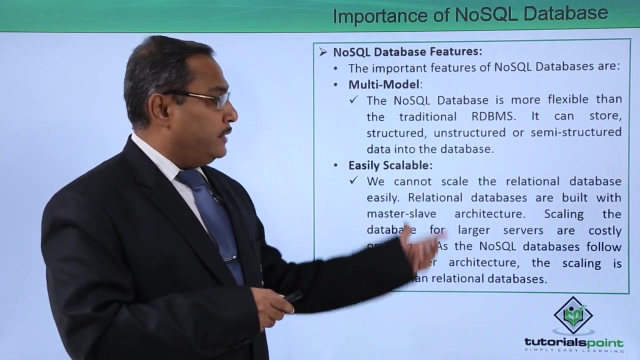 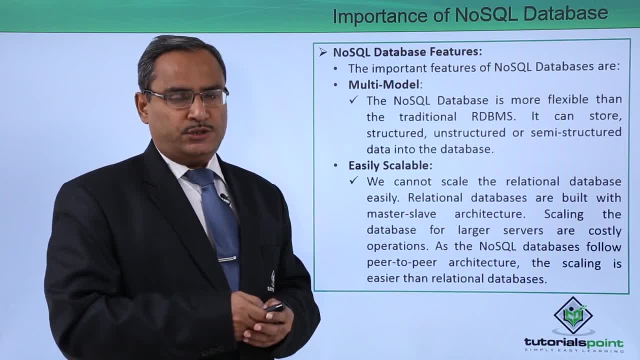 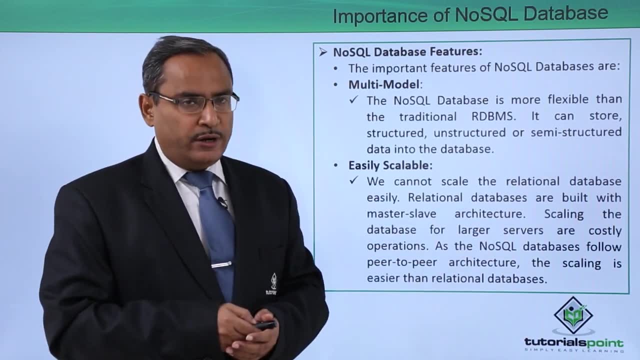 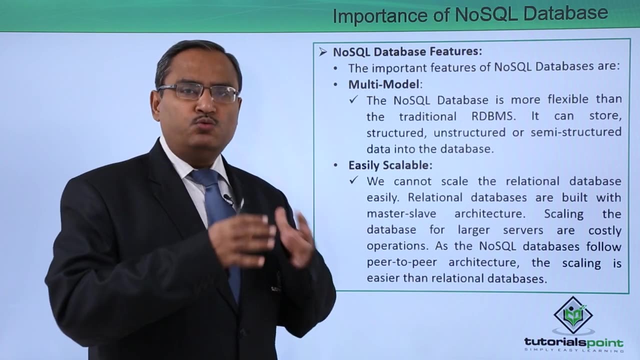 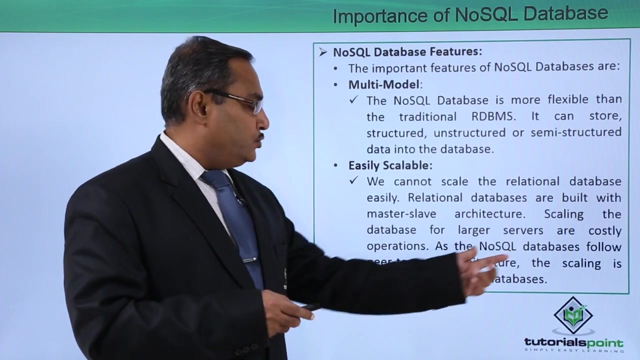